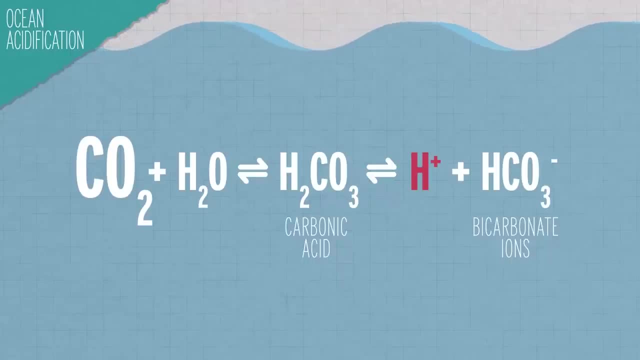 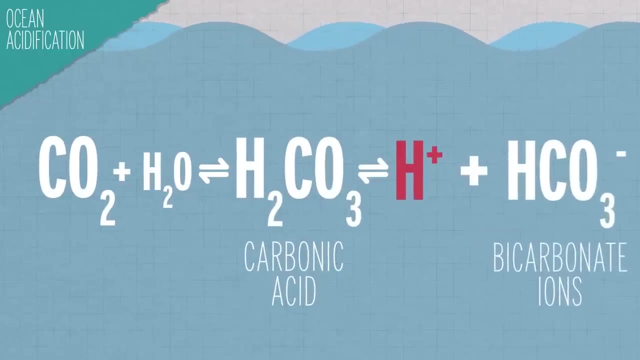 increasing its concentration. you're going to shift the equilibrium and the reaction is going to try and relieve the stress. It's going to do that by making more and more carbonic acid, trying to return to balance This response of a chemical system to stress like a change in. 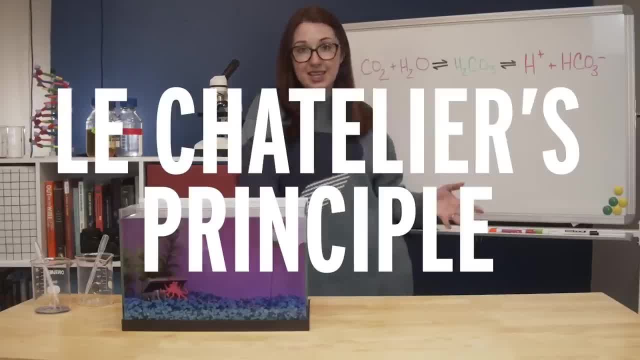 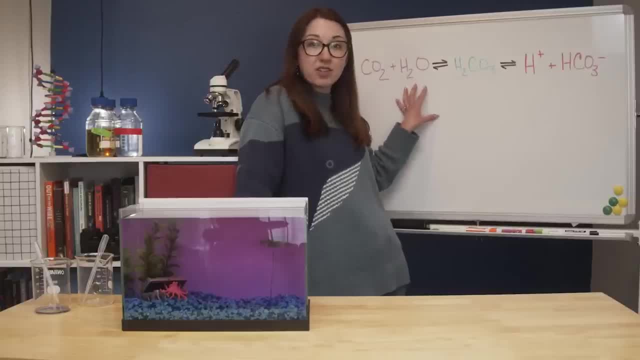 pressure or temperature or concentration is known as Le Chatelier's principle. Basically, as you get more and more CO2 on the left, it's more likely that it'll bump into these water molecules, react and then move the equation to the right. In the end, that's going to cause more hydrogen ions and a more acidic ocean, And this can be problematic for stuff living in the ocean, particularly shellfish and corals. They rely on carbonate ions in the water to build their shells, But the hydrogen ions react with the carbonate to form even more. 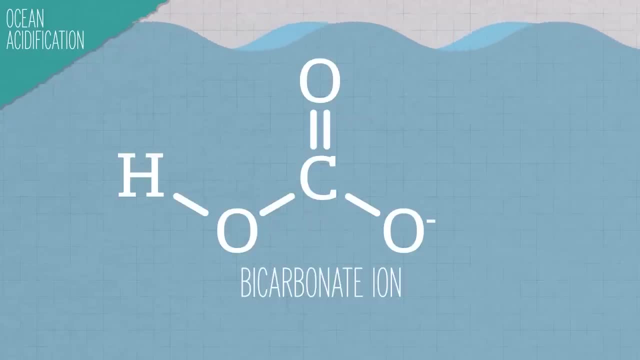 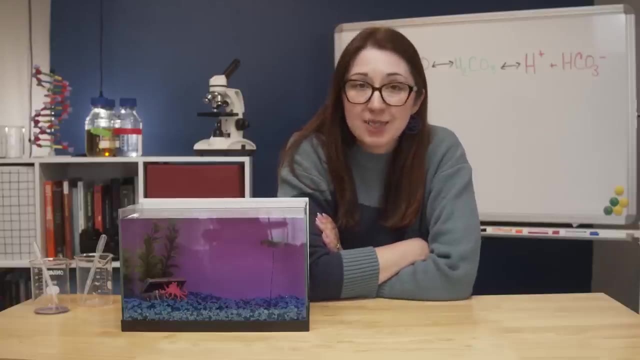 bicarbonate, reducing the amount of available carbonate for organisms to build their shells. The average ocean surface pH has declined by about 0.1 units since pre-industrial times, which works out to about a 16% decrease in available carbonate ions. But the main problem? 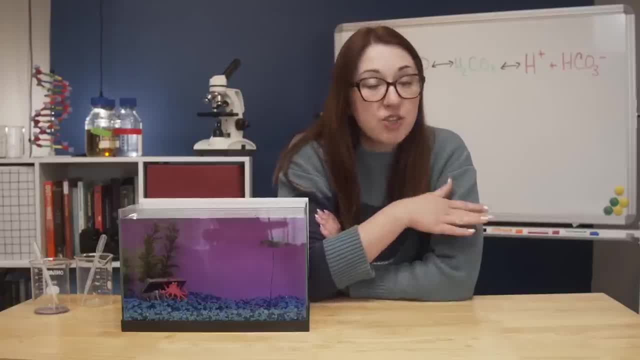 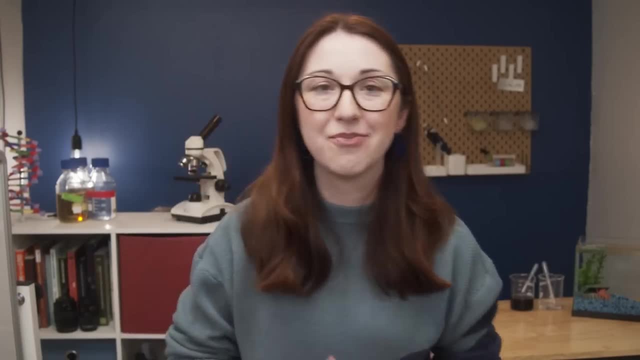 with ocean acidification isn't the shellfish, or even the impact on industries and communities that depend on shellfish to survive. We don't care about the shellfish. I mean, I do, I do, but The bigger problem is that the increased acidity also reduces the 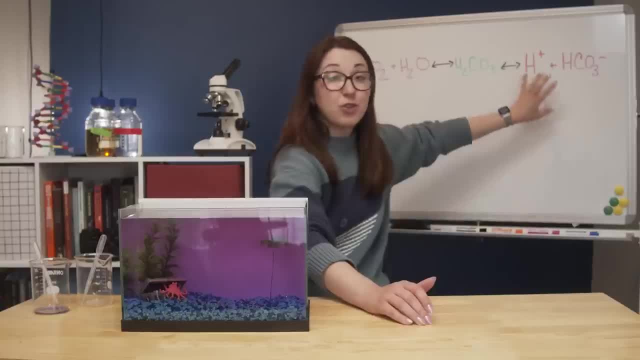 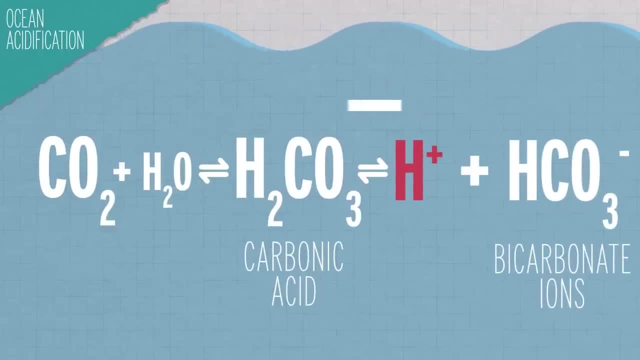 ocean's ability to take more carbon dioxide out of the atmosphere. You have more hydrogen ions over the ocean and the reaction wants to relieve this and get back to balance by pushing things out towards this section and you get more CO2 and H2O out And it would be really helpful if the ocean could keep absorbing more CO2, since there's already way too much up there and we are still cranking out more. Stopping our carbon dioxide emissions would be the actual solution, But, honestly, we have raised CO2 levels so much that, even if we did stop, we would still need to pull. 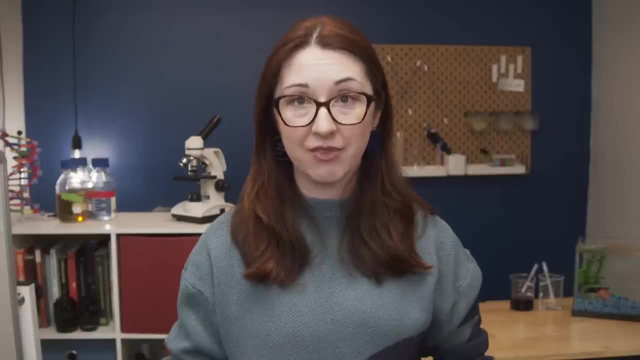 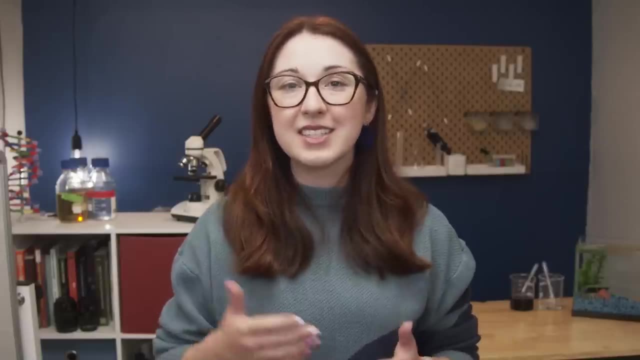 carbon out of the atmosphere to try and mitigate the negative impacts that climate change is going to have. This is all kind of a band-aid, but it is a band-aid that we really need to work. Reversing this acidification by alkalizing the ocean could help the shellfish reinvigorate the 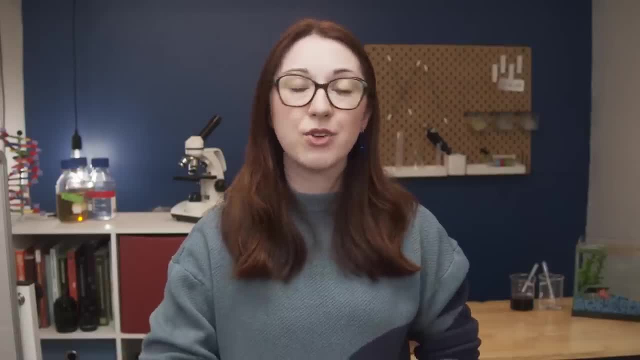 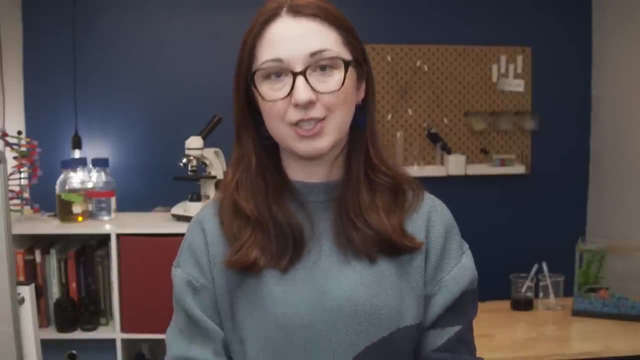 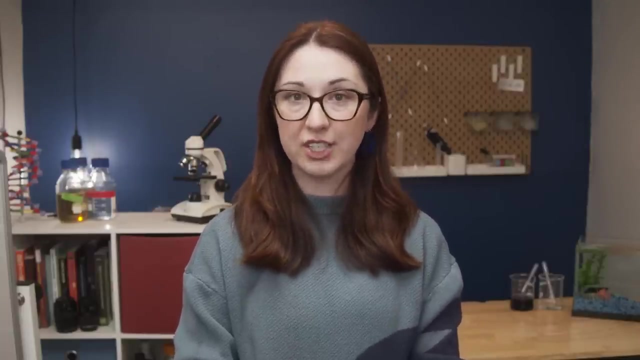 carbon dioxide absorption ability of the ocean and slow down the rising global temperature. So let's just raise that pH, right? Well, what we're talking about here is sometimes considered geoengineering. Geoengineering is the deliberate, large-scale intervention in the Earth's natural systems to counteract climate change. 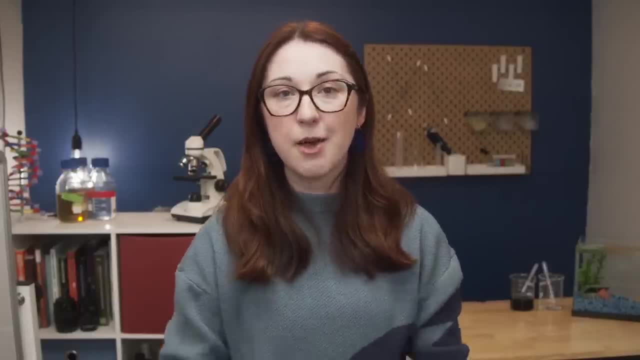 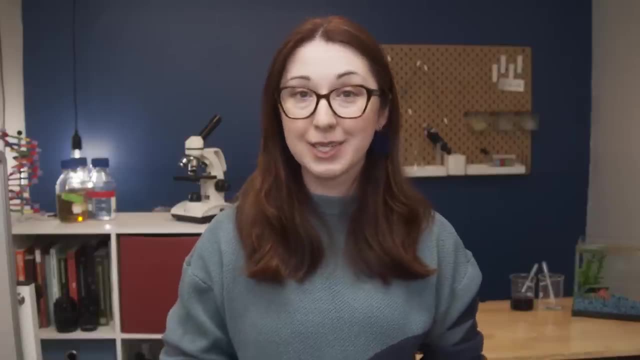 One of the most common types that people think of is solar radiation management, basically taking big shields or aerosolized particles to bounce the sun's energy away from us. There are really people thinking about trying that. Now the idea is that we've messed. 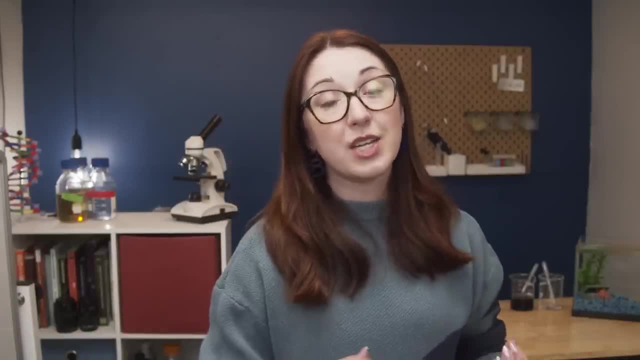 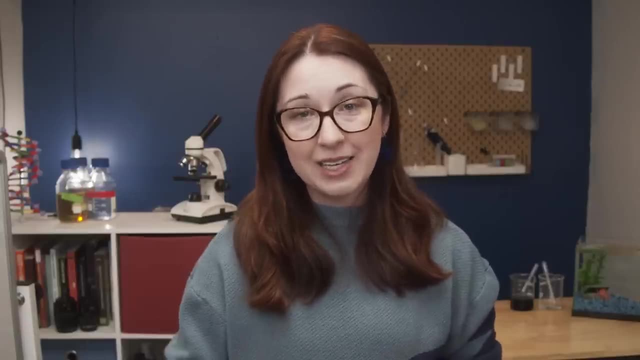 up the balance of the planet, so let's engineer it back And, as you can imagine, this is controversial. Proponents note that even if we stopped all CO2 emissions today, we have already changed the environment so much that effects would persist for years and years. 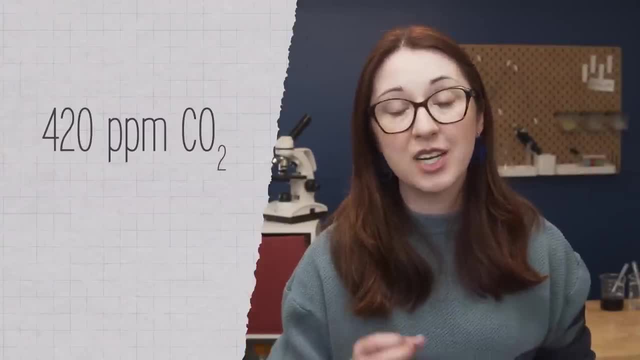 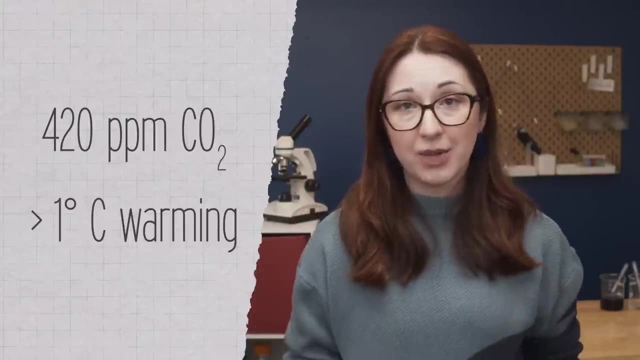 In fact, we've put about 420 parts per million of CO2 and other greenhouse gases into the atmosphere already, resulting in a full degree Celsius of warming, which is already having effects on our planet. So we really need to do something to help set the ecosystem back. 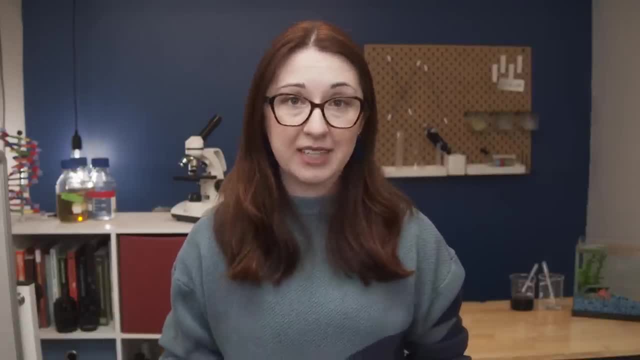 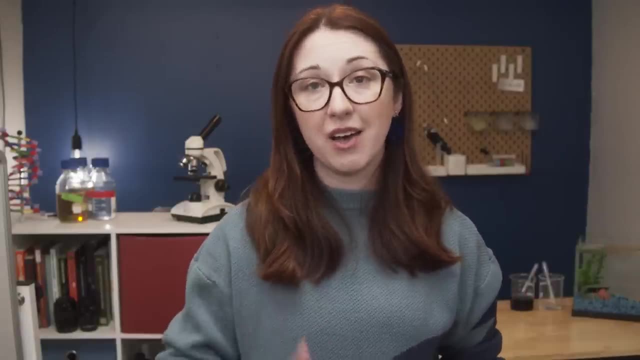 But critics point out that we clearly don't have a great track record of impacting our planet's climate and our efforts to fix it. that could be things like bouncing the sun's rays into outer space could have unintended consequences, Things like ecological disasters. 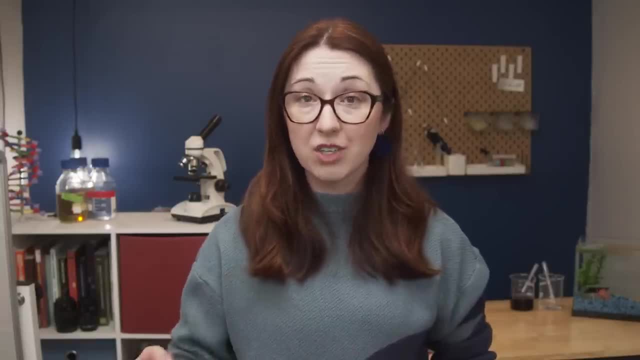 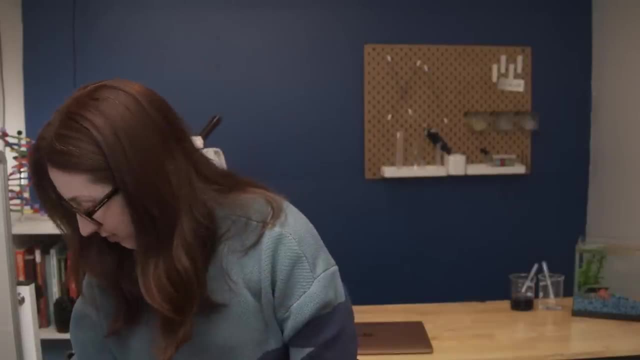 weather patterns that destroy the climate or economy of different parts of the world, the movie Snowpiercer, etc. I actually really love Snowpiercer. I don't want to love it, but it was cool. Ocean alkalinization is in some ways, geoengineering. Its overall goal is to use 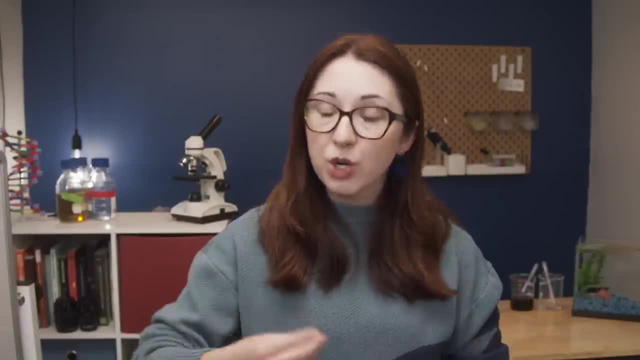 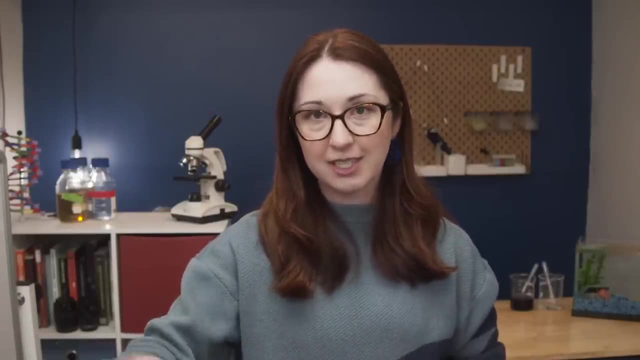 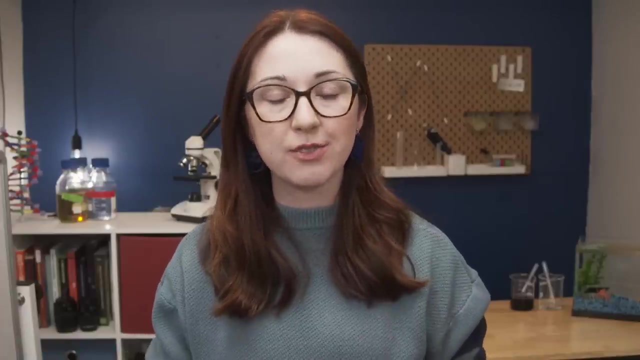 the ocean's ability to store carbon, to draw carbon out of the atmosphere. So it is a form of carbon removal. but we're also modifying the state of the ocean in the process, engineering that ocean. So I call it semantics. If we want to geoengineer our way to a less acidic ocean, why not start with Tums? Tums are mostly calcium carbonate. So what's going to happen is that that calcium carbonate is going to react with the hydrogen ions. That is going to, in turn, form HCO3, more of that bicarbonate as well as calcium. It's going to leave that calcium behind. 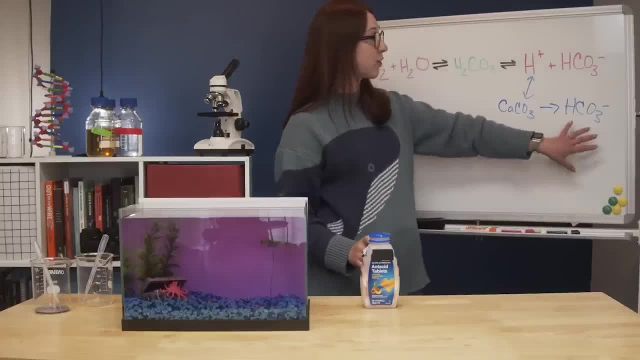 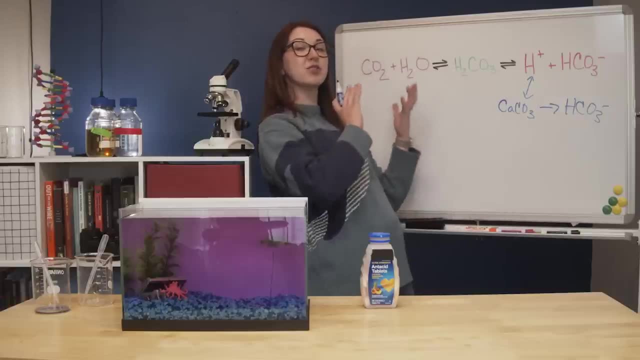 Now we don't really care about this. What we care about is the fact that this bicarbonate is now going to increase in concentration and we're going to push this reaction back. this way, It's going to relieve stress by now creating more of that carbonic acid and then more of the CO2, and 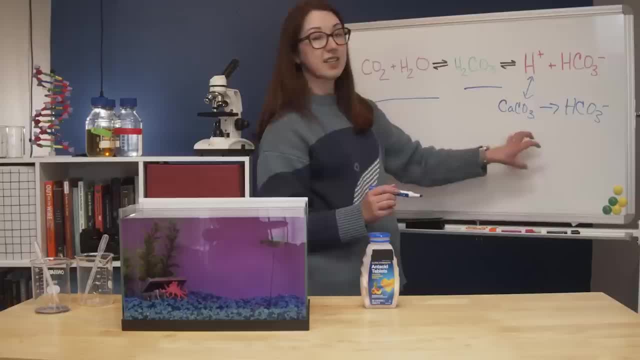 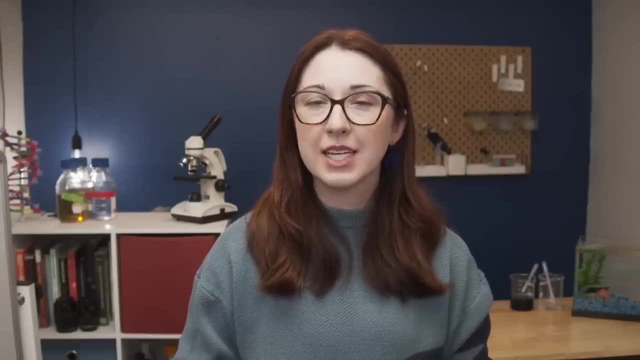 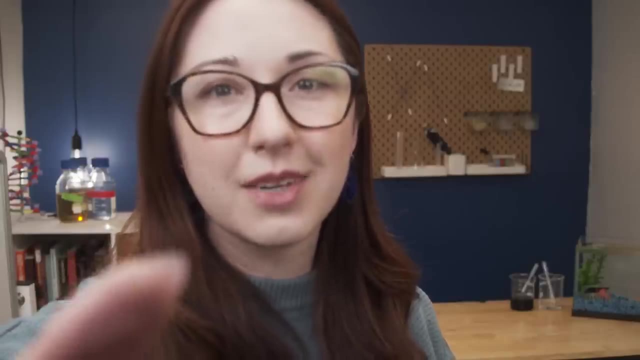 H2O. So this calcium carbonate is going to reduce that hydrogen ion concentration and also push this reaction back. this way Can you have a singular tum? Take a tum, I think. I think I think of it as Tums A Tums. But the CO2 byproduct from calcium carbonate isn't ideal here, So some researchers are 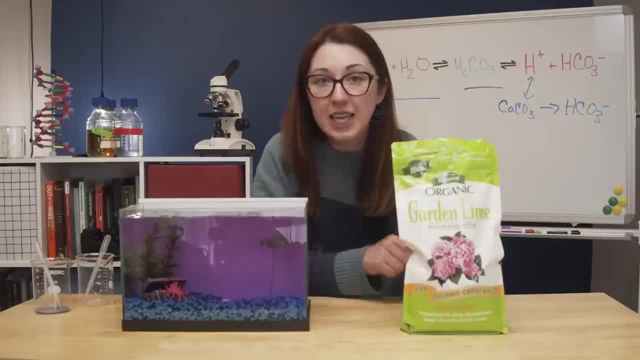 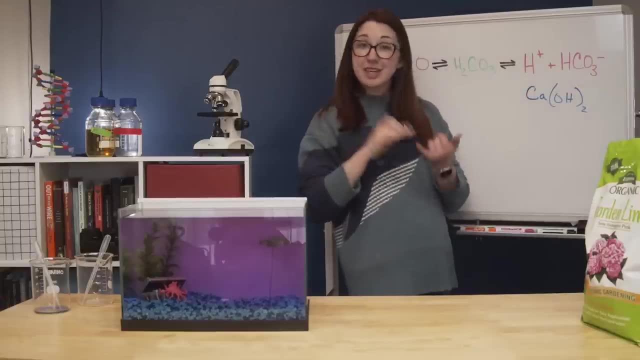 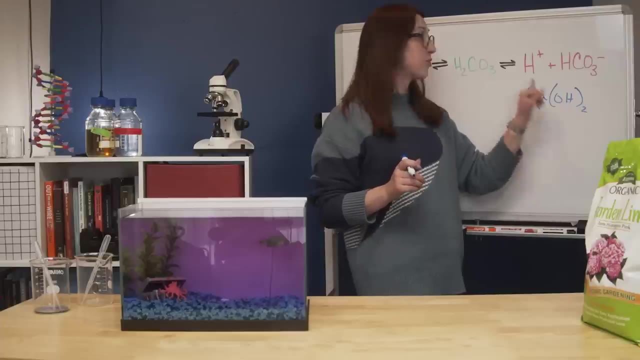 trying it with lime instead. Lime is mostly calcium hydroxide, C-A-O-H-2.. It's commonly used in both cement and corn tortilla production and it is really great at neutralizing acidic solutions. These hydroxide ions can react with the hydrogen ions, creating water, pushing the pH up, because 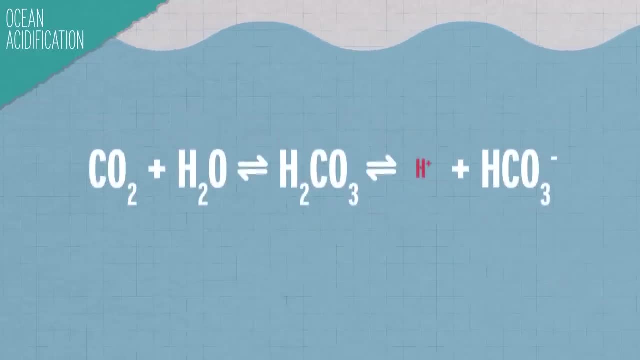 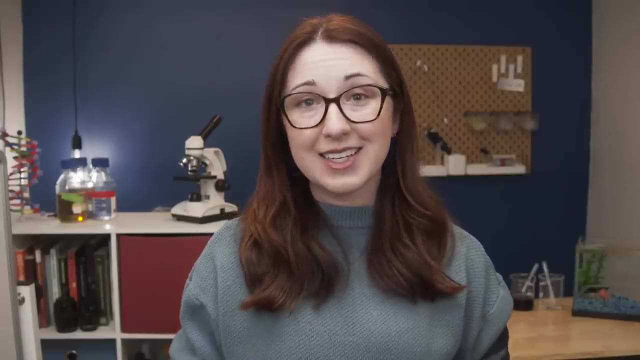 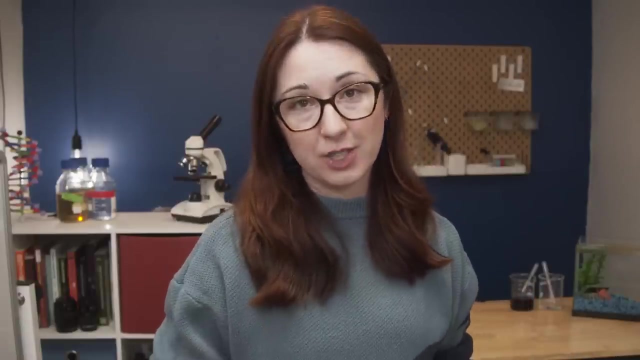 we're reducing the concentration of these hydrogen ions, allowing us to pull more CO2 out of the atmosphere. This way, Early tests look like they are in fact reducing the acidity in areas near releases of lime. For example, one trial in an estuary saw a decrease in dissolved CO2 of 70 parts per million. 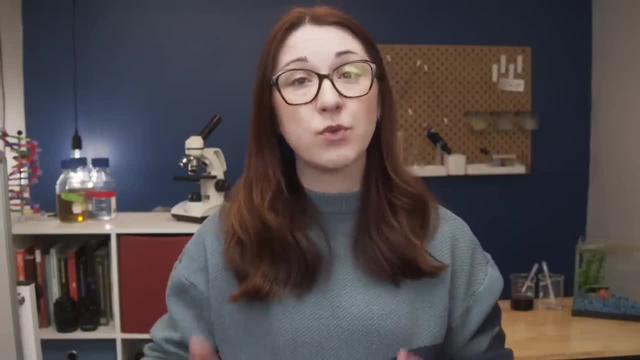 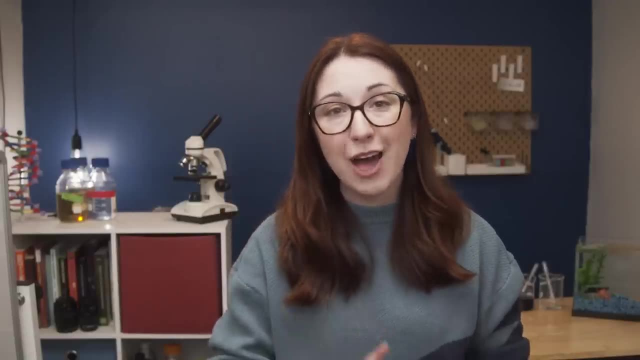 which is a surprisingly significant amount. Proponents admit that we really have to target areas in the ocean like this, where the alkalinity experiments would have the greatest effects. They also note that it matters how the air and ocean water interact. If your alkalinized water circulates away from the surface too fast, it won't have time to re-equilibrate with the air above it, And that exchange time can vary based on location from days to months. But there are some big buts here, both with ocean liming in particular. 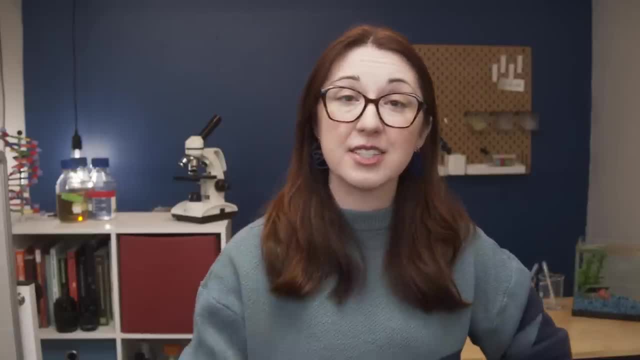 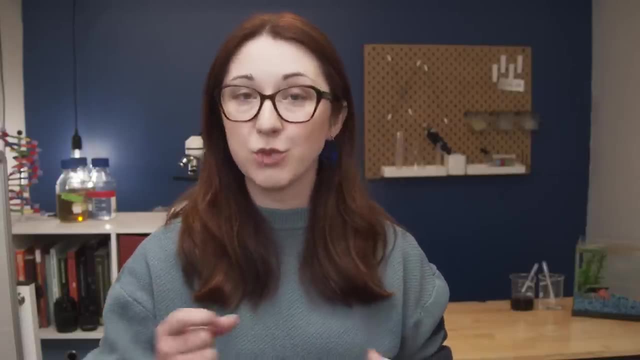 and with ocean alkalinity enhancement in general. So first for liming: where are we getting all that lime? Lime comes from limestone. You first have to mine the limestone, which gives off CO2, and then usually heat it to get lime, which then also gives off CO2.. One estimate suggests that it would take 1.4 to 2 hours to mine the limestone And that would take 1.4 to 1.7 tons of limestone to sequester 1 ton of CO2. And turning that amount of limestone into lime could give off about 1 ton of CO2.. Now that CO2 would be produced in a controlled manner and could ideally be directly captured and sequestered. But we would need a whole system in place for that too. We would need green energy, carbon capture and a whole lot of money to make it work. 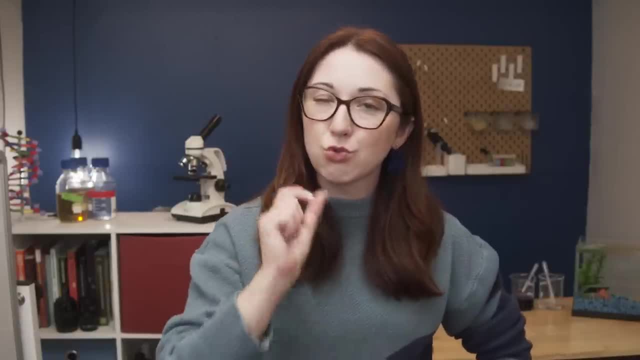 The other thing here that became clear as I read all of these papers and that I think is really important to understand, is that all of this stuff is going to be used to make lime. All of these estimates and analyses have huge numbers of variables. 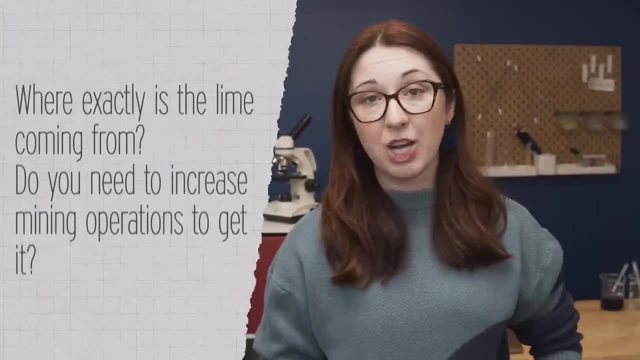 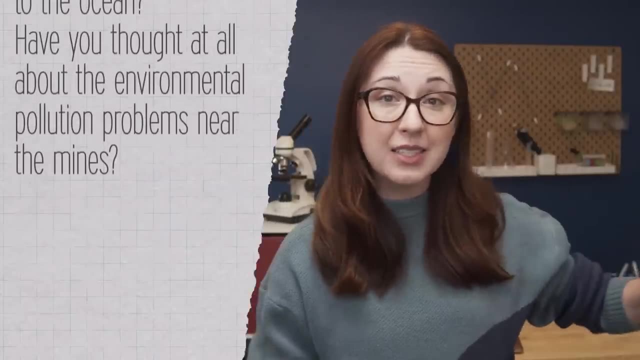 Things like: where exactly is the lime coming from? Do you need to increase mining operations to get it? How are you shipping it to the ocean? Have you thought at all about the environmental pollution problems near the mines? What about any ecological effects to the surrounding aquatic? 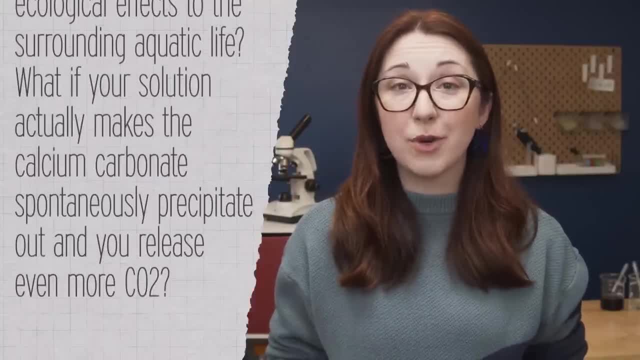 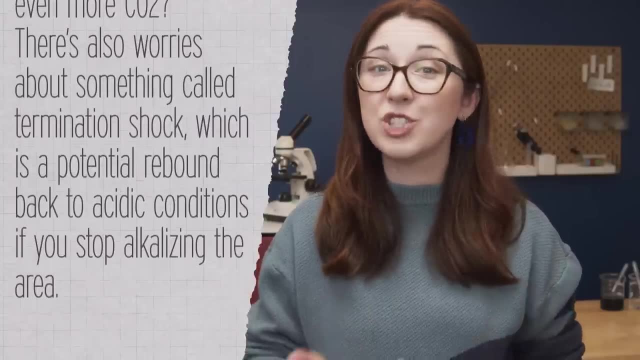 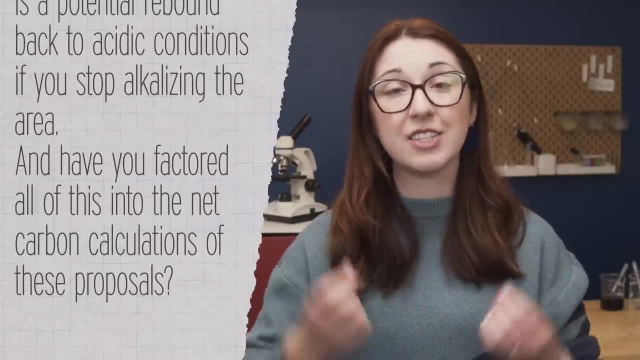 life when you dump in a bunch of lime, What if your solution actually makes the calcium carbonate spontaneously precipitate out and then you release even more CO2?? There's also worries about something called termination shock, which is a potential rebound back to acidic conditions if you stop alkalizing the area. And have you factored all of this into? 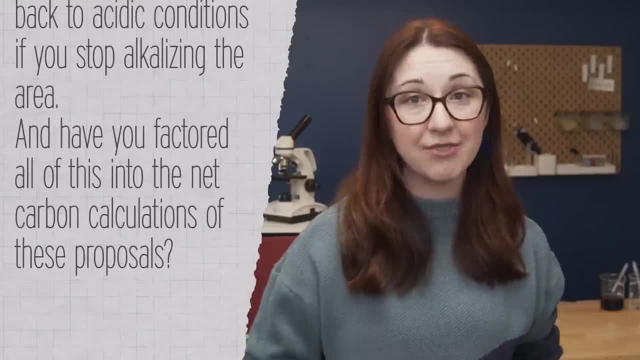 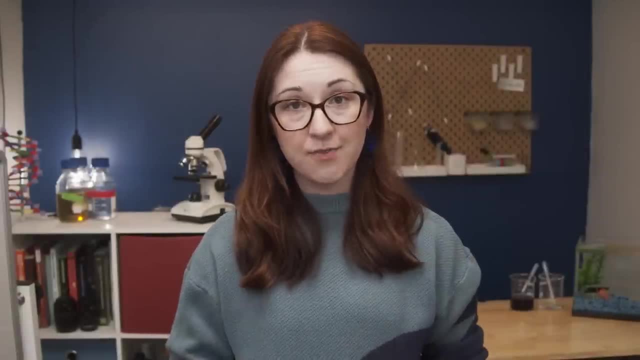 your net carbon calculations for your proposal, creating a lifetime assessment of your solution. Here's the thing. This isn't to say that any of these are deal breakers. It is just a lot to consider, and good researchers are considering all of it. 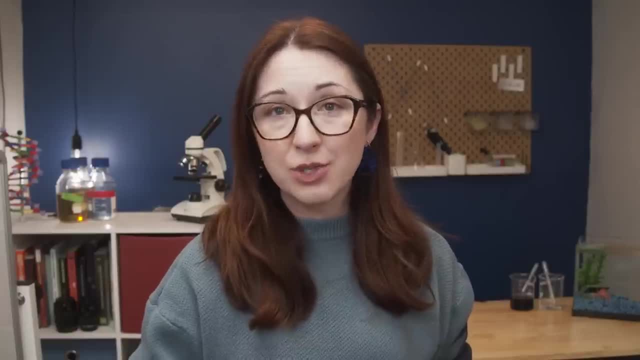 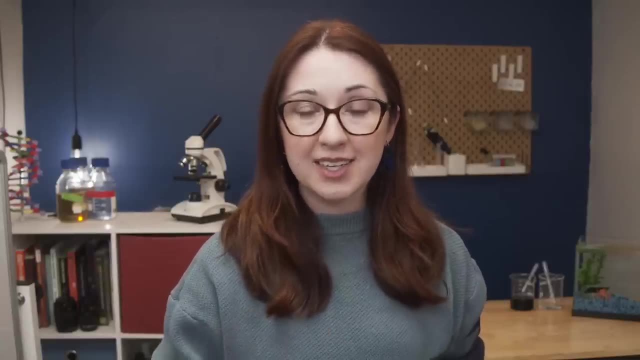 And that's why a different analysis which looked at what it would take to continuously alkalize the ocean for the next three hundred and eighty years, putting us at the nice even year of twenty four hundred, came up with a cost estimate between one and several trillion dollars, USD each. year. The difference between one and several isn't large, but the difference between one trillion and two trillion is gigantic. So these estimates have huge ranges in terms of cost, energy needs and CO2 output. So there's another method of ocean alkalinization that's getting some press. 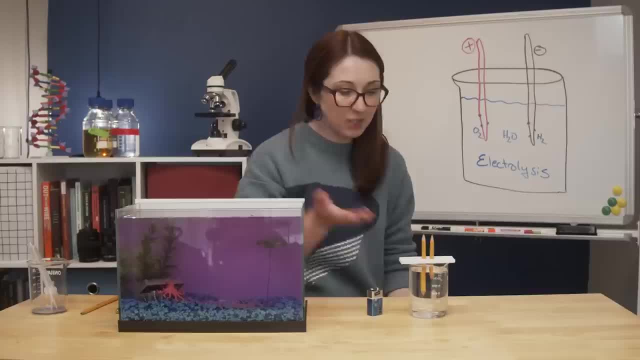 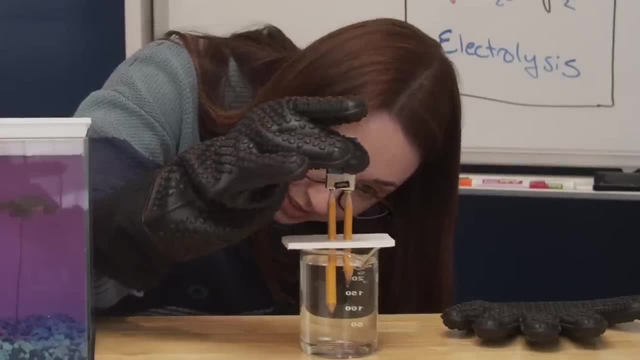 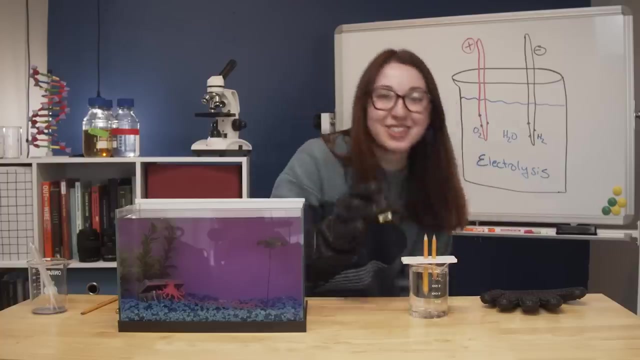 and investment money: Electrolysis, Seawater, a couple of electrified plates. Honestly, it is not included in this, but if you want to make sure that you don't damage the ocean, then don't. Oh yeah, Oh my gosh, it's working. That's so cool. I love when science works. Thing is, you would need a lot of these plants to really make a difference. One of these startups is planning the launch of a commercial plant in the next year that aims to pull the equivalent of the annual carbon emissions of twenty five thousand individuals out a year, And that's great. 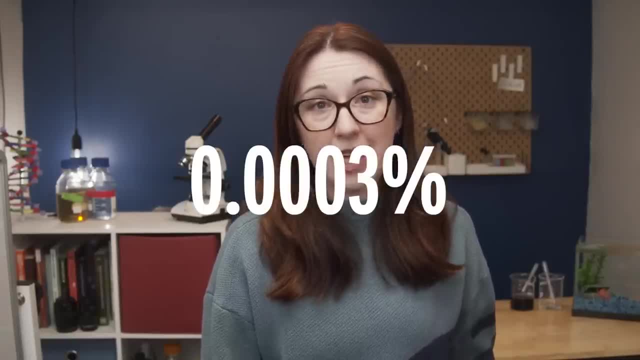 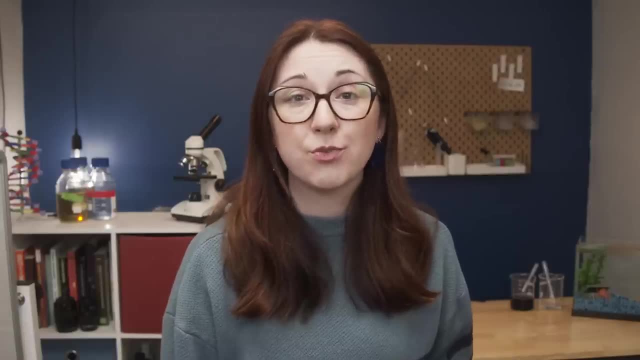 but it is point zero, zero, zero. three percent of the world's population, like the liming, the energy to actually do the electrolysis would have to come from a green or renewable source, to make sure that it wasn't producing more CO2 than it was removing. And I know that I am being a huge downer here, because we all want these solutions to just work. It would be really helpful if these plants just snapped on and they solved all the issues we're having, And certainly there are lots of people investing in them through grants and VC money and carbon. 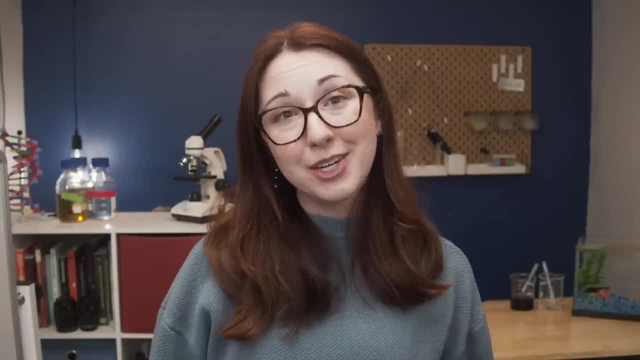 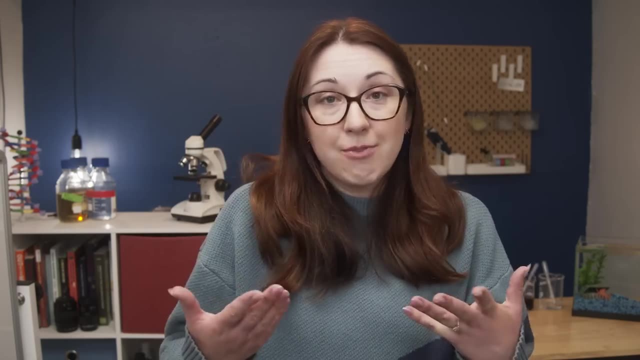 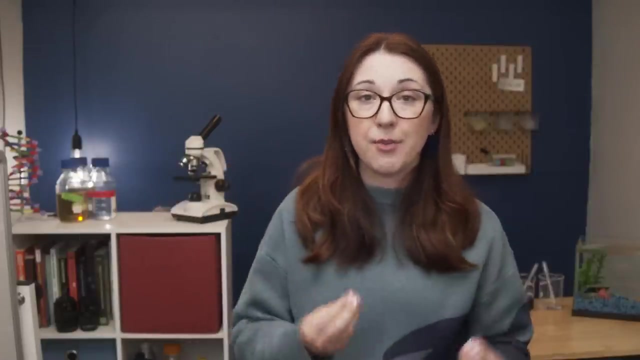 credits to try and get them there. Yeah, did that last one perk your ears up? Many of the startups in this space are selling carbon credits based on their technology. You give them X amount of money and they'll pull Y amount of carbon out of the air so that your airplane, or whatever, can put Y. 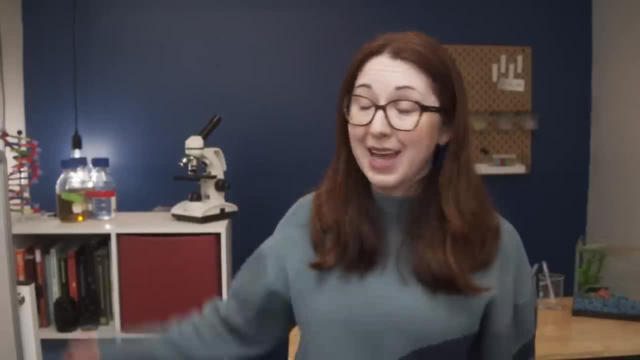 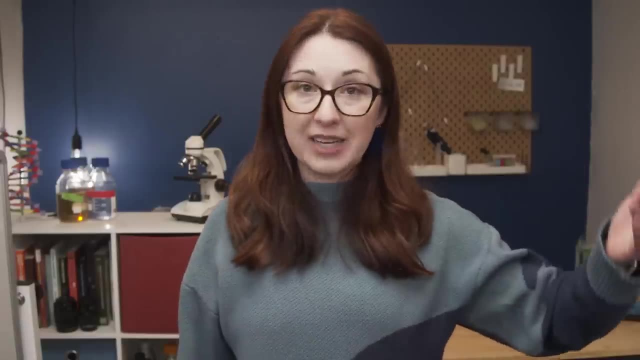 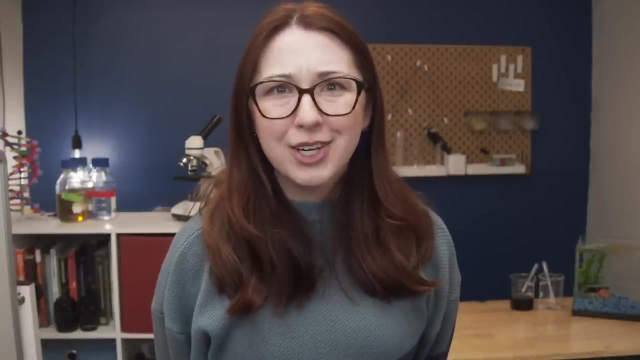 amount of carbon back into the atmosphere. But you can slap a carbon neutral sticker on it, And some of these companies are selling carbon credits out into the future based on what they expect to be able to do down the line. So your next five years of carbon emissions are covered. And what if those startups which are